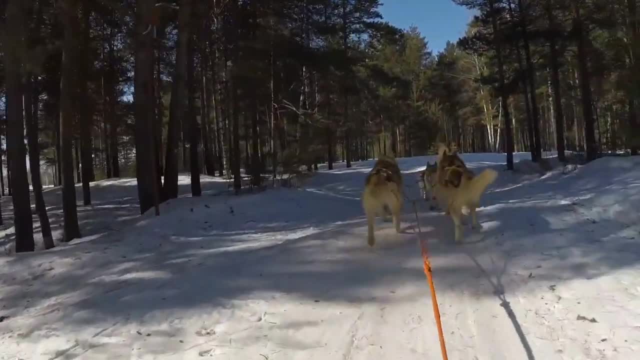 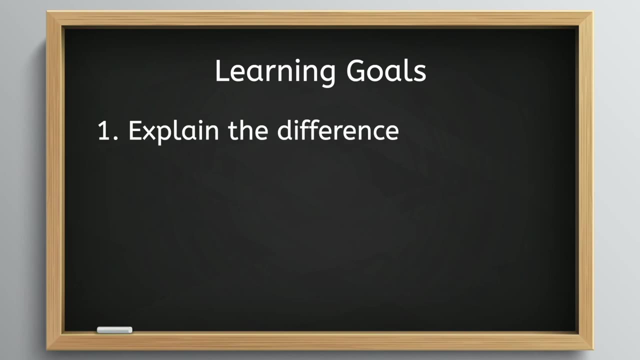 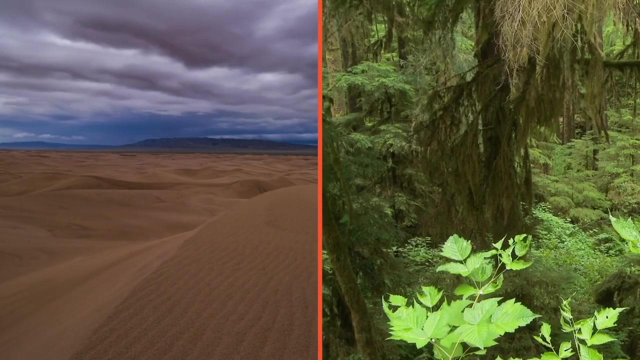 our lives, both in the here and now and over long periods of time. So today we'll be exploring those phenomena with the learning goals: explain the difference between weather and climate and explain how weather and climate shape human behavior Right off the bat. it's important to note that weather and climate are not the same. 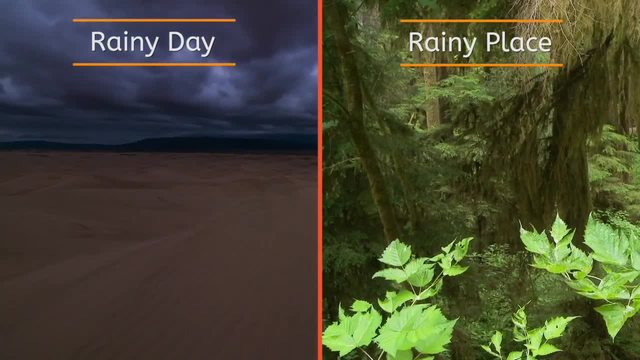 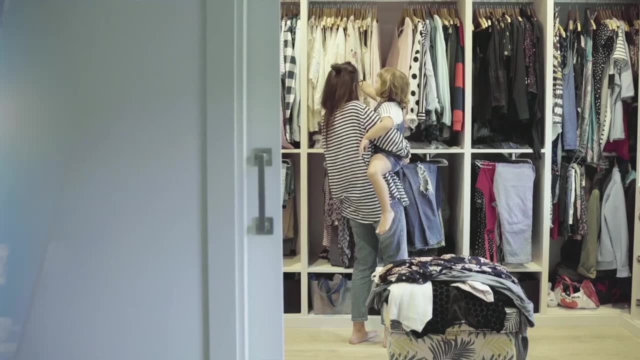 thing. An easy way to remember. the difference is this: Weather determines what you might wear on a particular day. Weather determines what you might wear on a particular day, While climate determines what clothes you keep in your closet. See, weather is the state of the atmosphere in a specific location at a specific time. 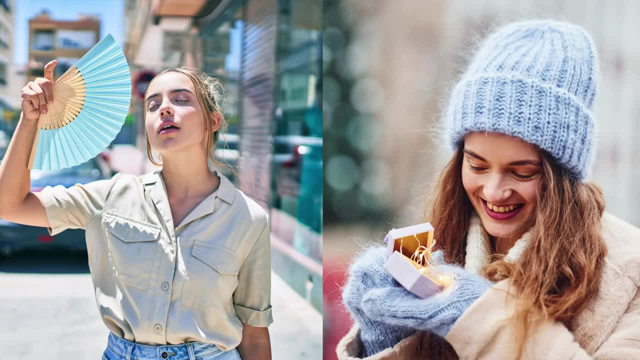 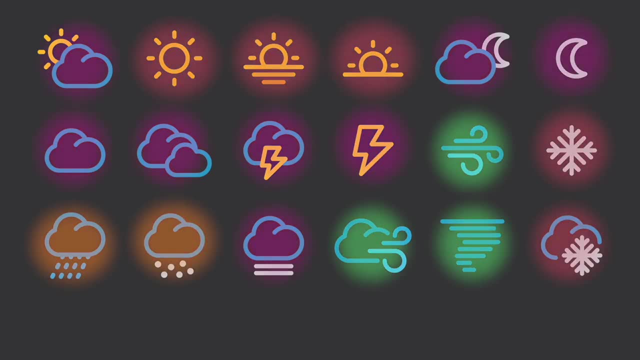 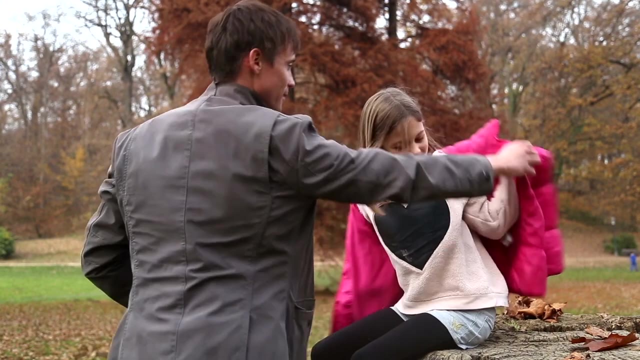 Is it sunny or cloudy? Is it warm or cool, Windy or calm? Precipitation, the temperature, the wind and other in-the-moment phenomena are weather events. The weather does impact the way we behave. It shapes small decisions we make. 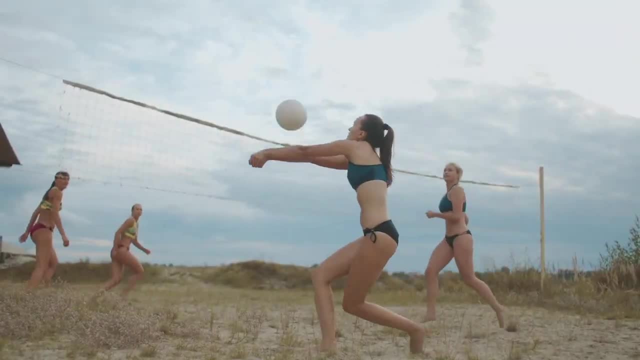 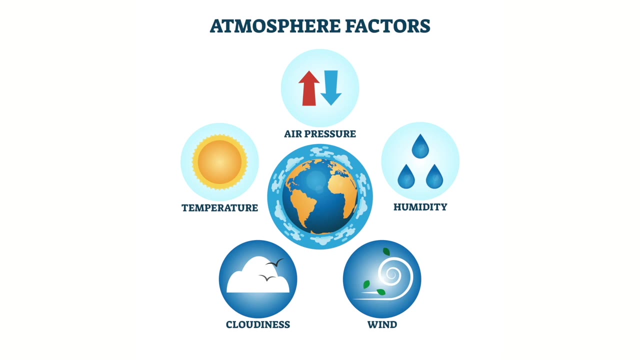 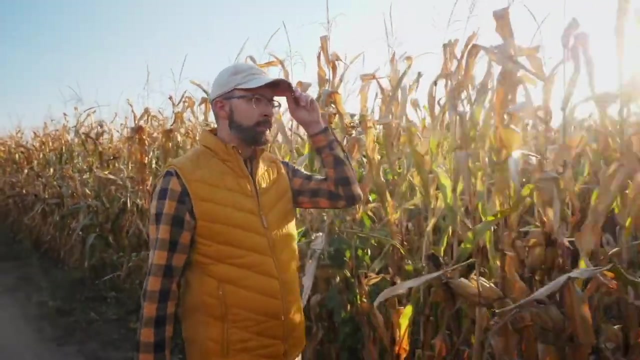 Like what we do, What we wear Or what activities we do over the weekend, But because there are many factors that determine the specific state of the atmosphere at any given moment, the weather can be extremely difficult to predict And the consequences for not knowing what the weather will be can be severe. 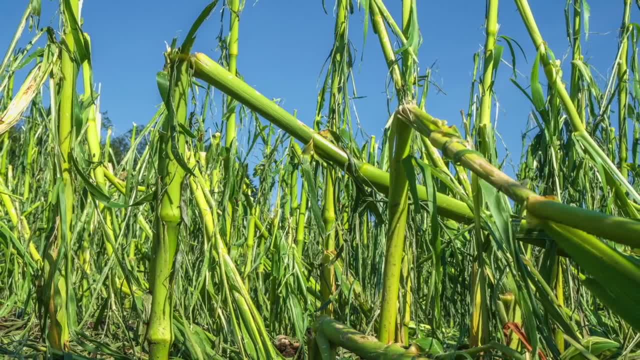 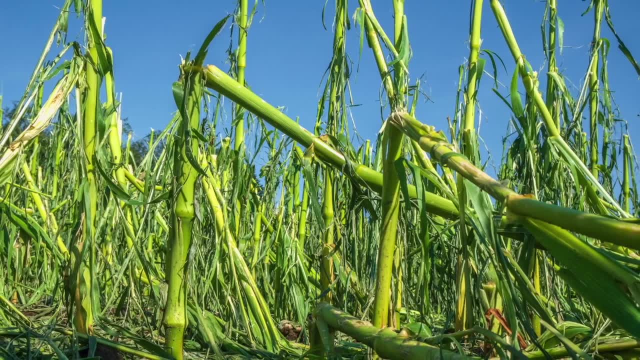 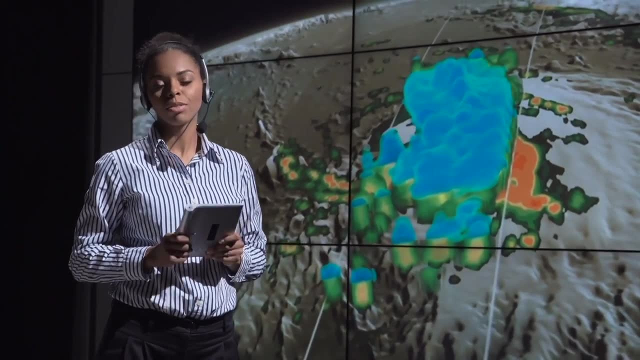 Weather events can have a big impact on people in a particular area. A hail, storm or heavy winds might destroy crops and cornfields, damaging the food supply and the local economy, Or a tornado can be devastating to local infrastructure. That's why TV meteorologists can make a career out of forecasting what will happen. 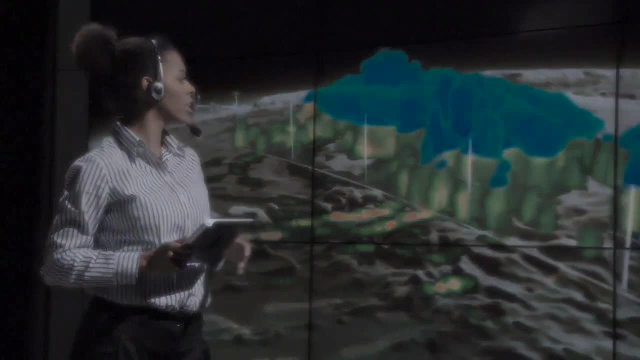 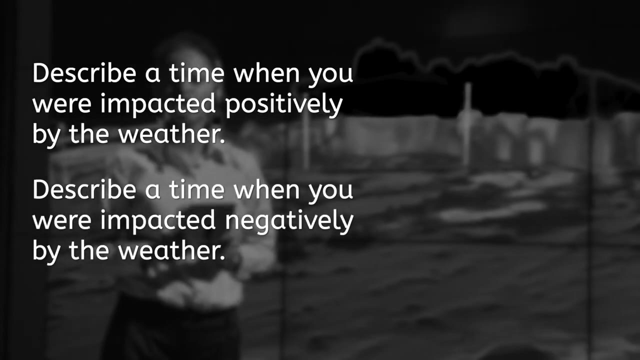 in the next few days. We need to know. Can you think of a way in which you were positively impacted by a weather event? What about a time when you were impacted negatively? Take a second to respond to the first two questions in the lesson guide. 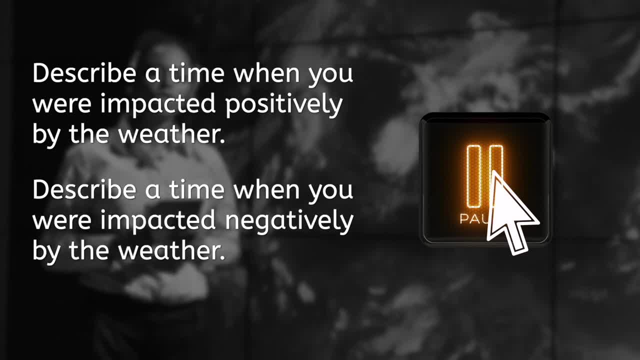 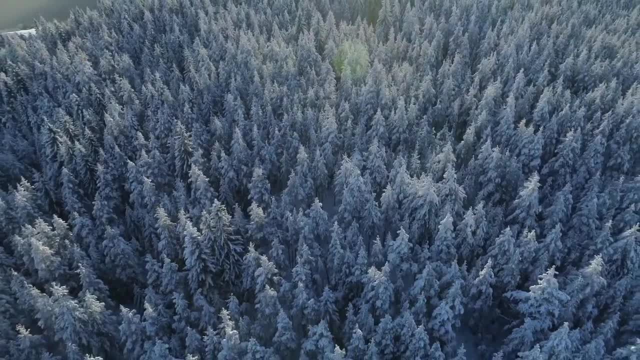 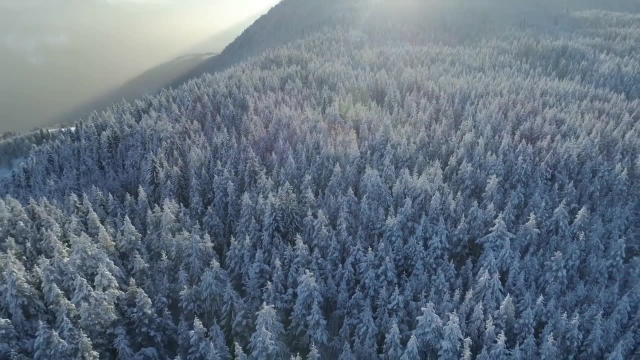 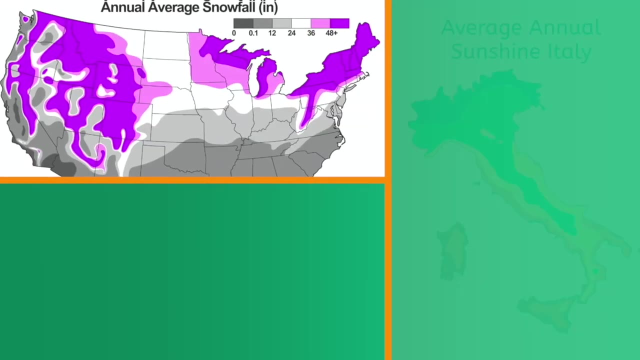 If you had a bad day, then you can't play. Climate, on the other hand, is not a day-to-day concept. The climate of a location refers to average weather conditions over a long period of time, like seasons and years. How many inches of rain or snow will an area get this year? 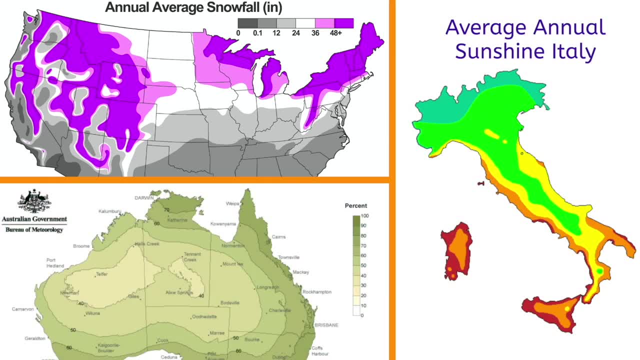 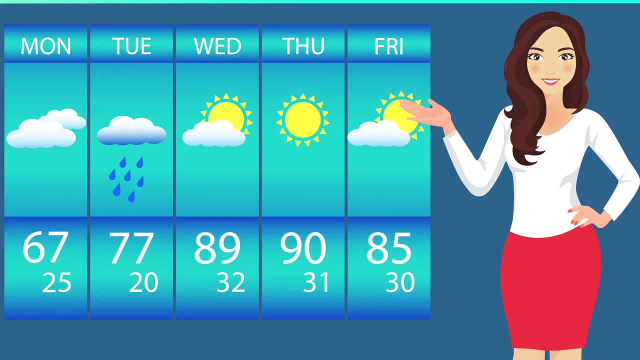 How many hours of sunshine will there be? Is it usually humid or dry? Changes to weather are extremely common And although they can be unfair, they are often even more important than changes to be unpredictable. the fact that they will happen is expected. Egypt has its rainy days despite. 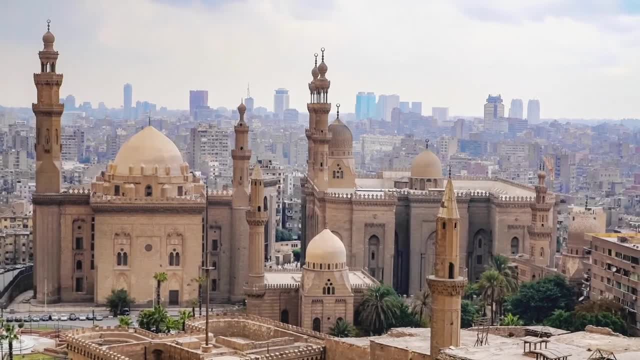 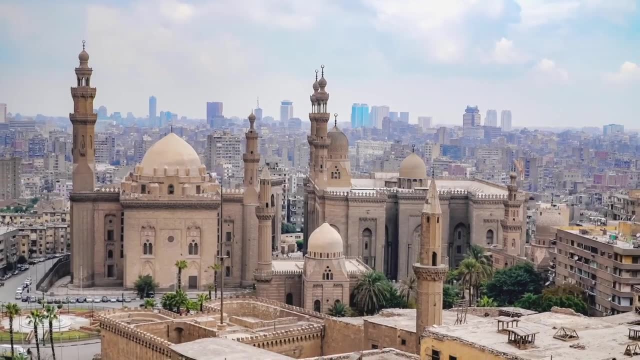 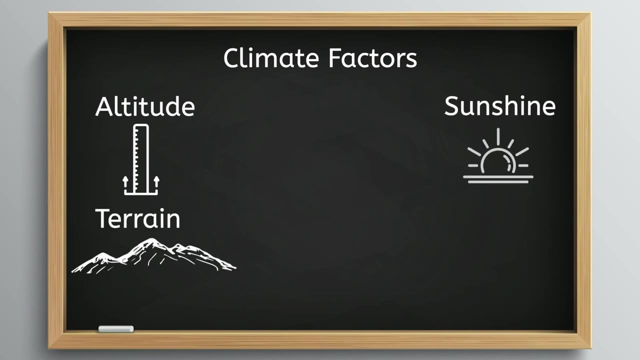 being a generally dry place, Changes to climate do not generally occur very quickly. Even though Egypt gets rain, it's still going to be hot and dry. for the most part, That's because climate is dependent on things like altitude, terrain, sunshine, latitude and nearby bodies of water. 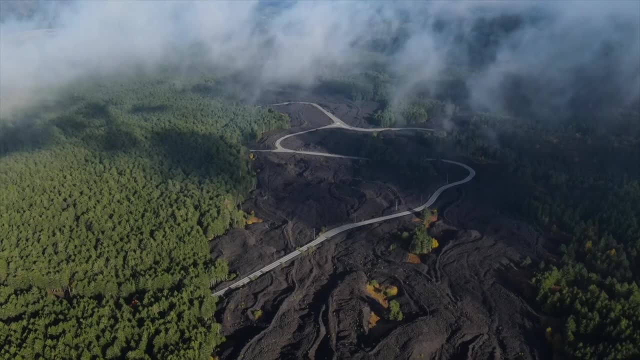 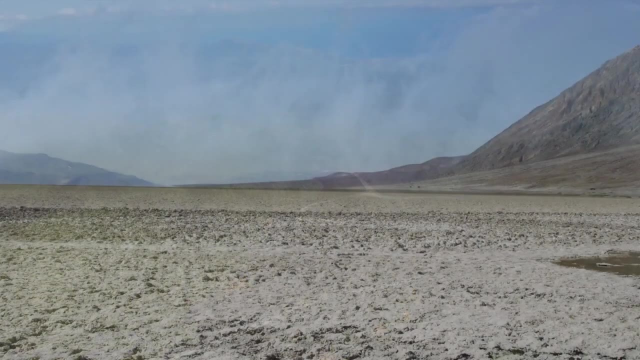 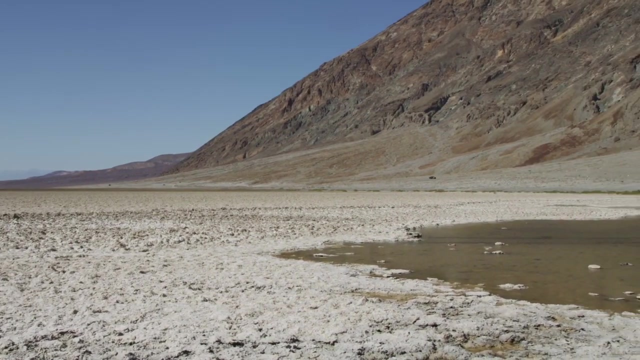 If the conditions of a place change, like if a volcano erupts and an ash cloud blocks most of the sunlight for a few months, climate changes may occur. But more often than not, climate changes occur when a huge lake dries up or as wind and water erosion change the terrain in an area. 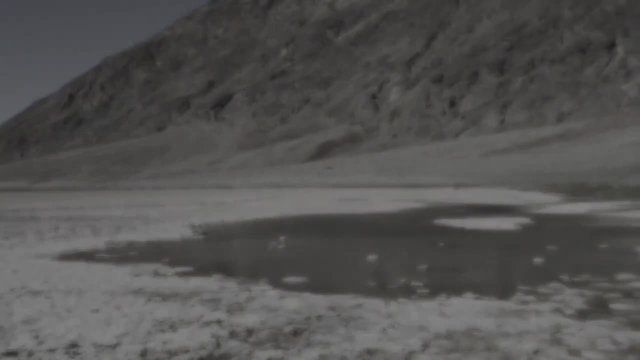 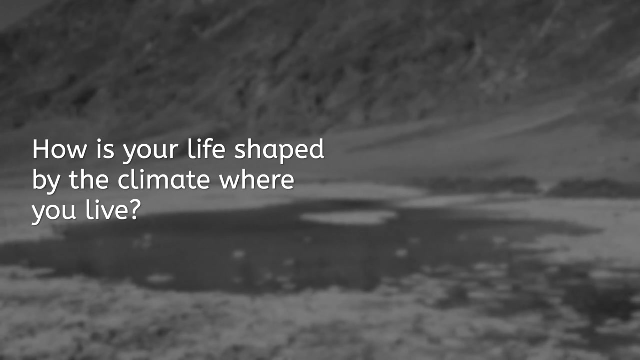 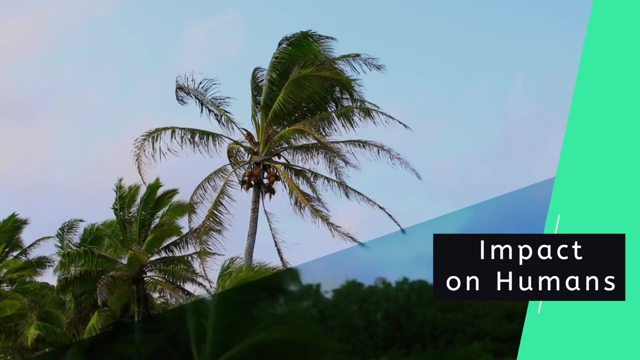 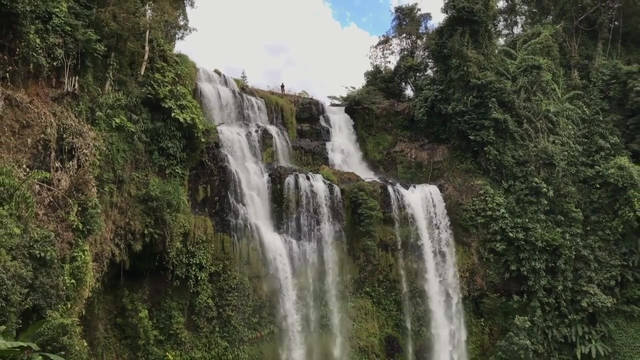 and those things take a long time. Okay, explorers, time to show what you know. How is your life shaped by the climate where you live? Pause the video to answer in your PDF If weather events were impactful because they may cause harm or disrupt everyday life. 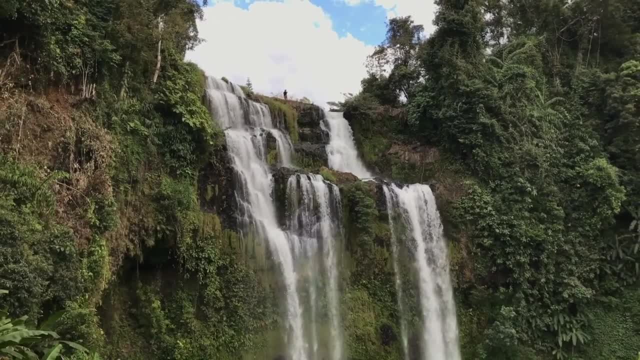 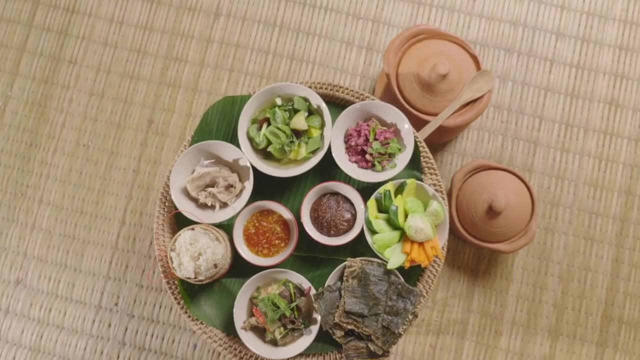 climate has much larger impact because it shapes everyday life. For most of human history, people have only been able to eat food that has grown locally, and what grows near you is dependent on climatological factors like how much rainfall you get and how much water you drink. 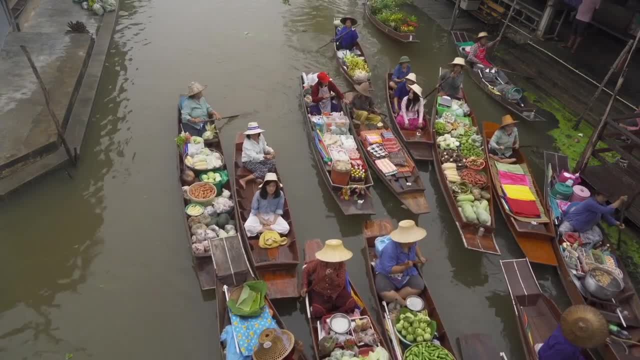 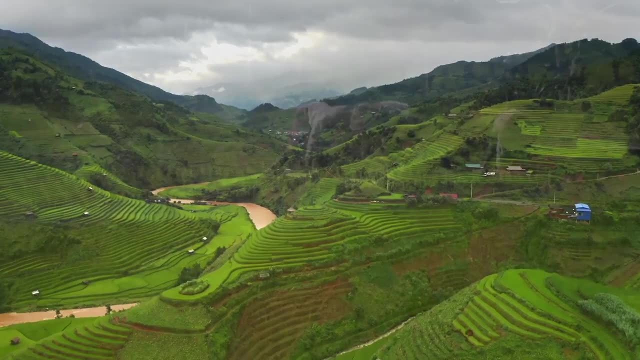 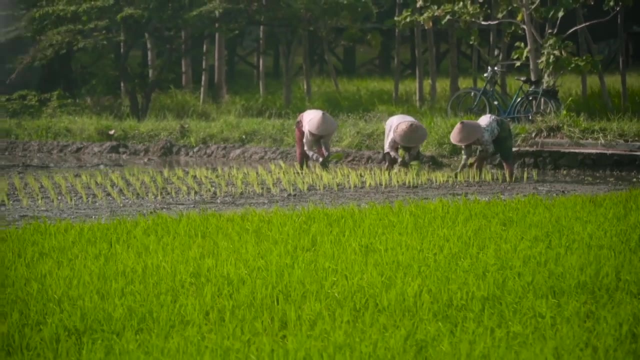 And how harsh the summers and winters are. Climate conditions in most parts of Vietnam are perfect for growing rice. A blend of climate, terrain and soil composition has made rice a staple in the diets of Asians for centuries. But people living in the Sonoran Desert of North